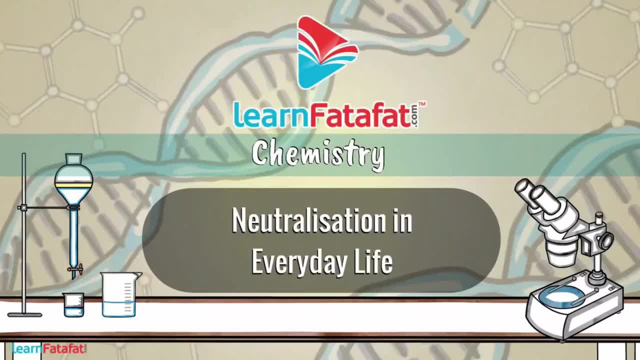 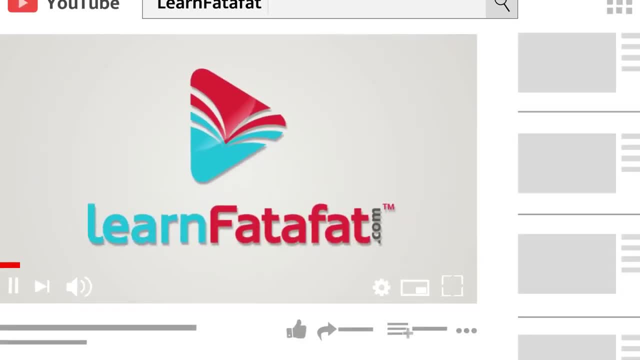 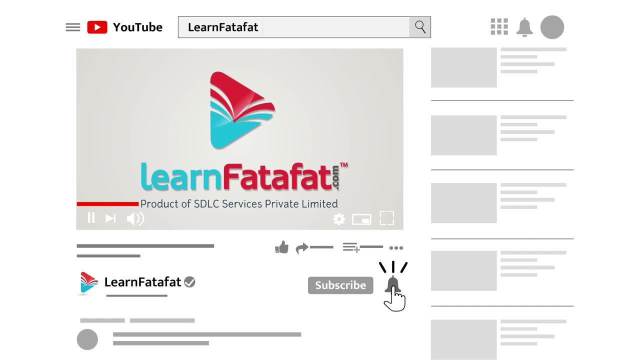 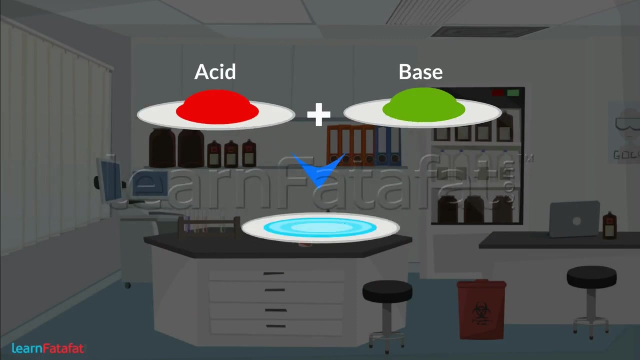 The reaction of acid and base so as to neutralize each other's effect, producing salt and water is called neutralization. 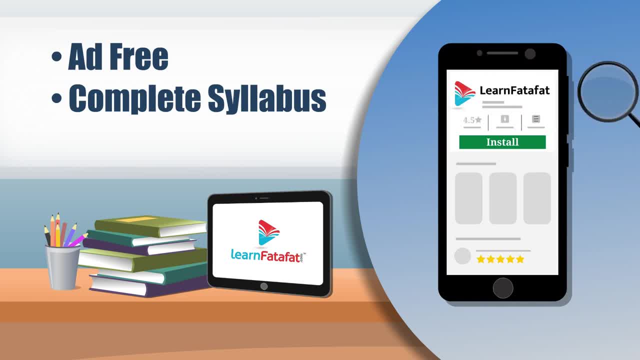 Watch ad-free and complete syllabus on Learn Fattah Fatt Android app. Download the app now. 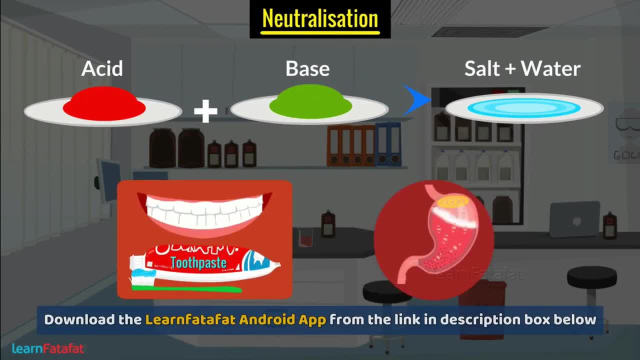 Knowingly or unknowingly, there are many neutralization reactions happening in our daily life. Let's understand some of them. 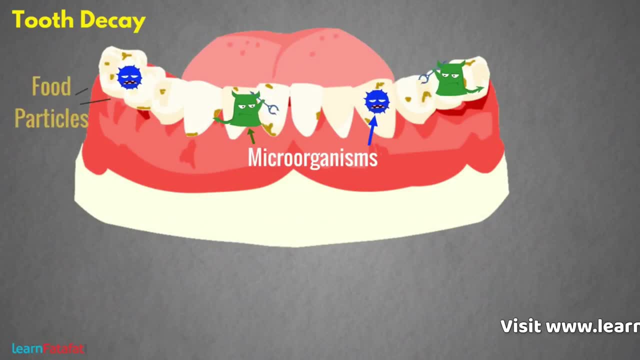 Tooth decay. Microorganism act on food particles in our mouth. Due to which, there is formation of acid. It acts on tooth and thus results in tooth decay. 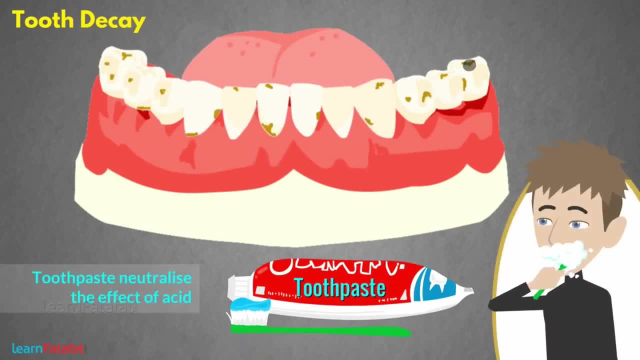 Toothpaste is used to neutralize the effect of acid and thus preventing the tooth decay. 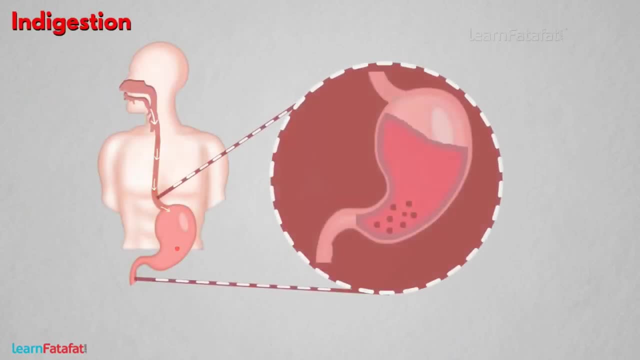 When we eat food, it goes in stomach. Here, the hydrochloric acid produced in stomach acts on food to digest it. 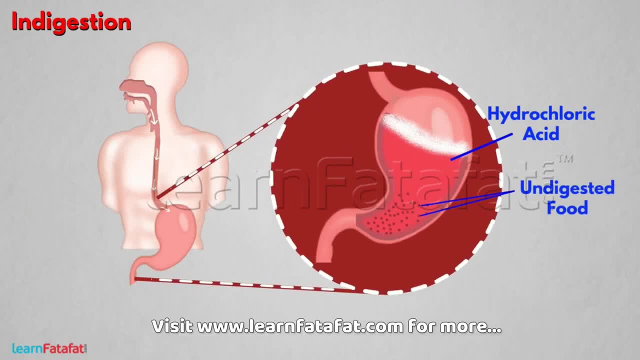 However, sometimes our body does not digest the food and we feel fullness in our stomach or burning sensation in upper stomach area above it. It causes pain. This condition is called indization. 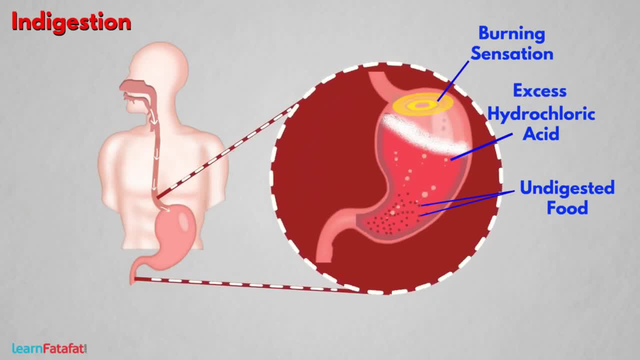 It happens due to excess of acid in our stomach. To relieve indization, we take medicine consisting of base such as magnesium hydroxide which is also called magnesium hydroxide. 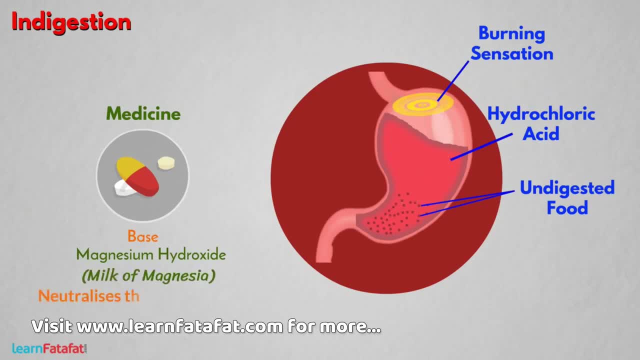 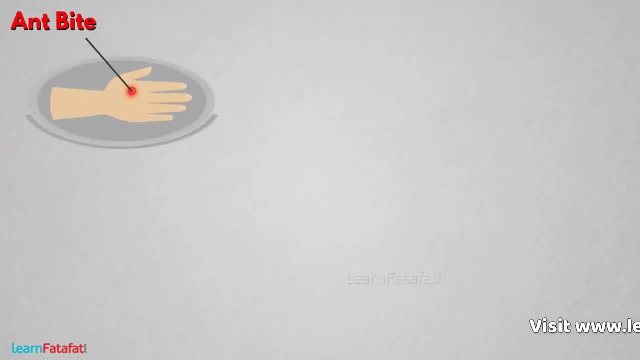 Ant bite Ant bite is very painful because during the bite ant injects an acid called formic acid in our body. It causes burning sensation and pain. 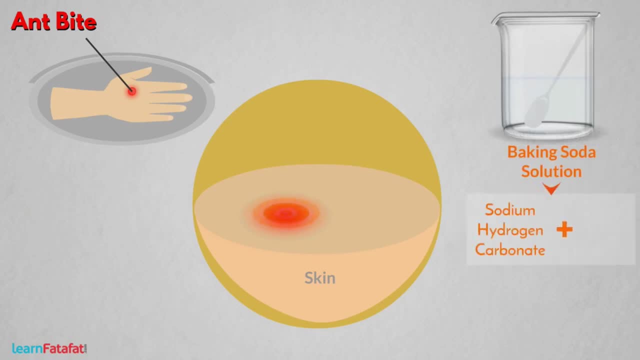 If we make mixture of baking soda that is sodium hydrogen carbonate with water and apply it on the bitten area, we feel relieved. It is because the base that is baking soda neutralizes the formic acid.